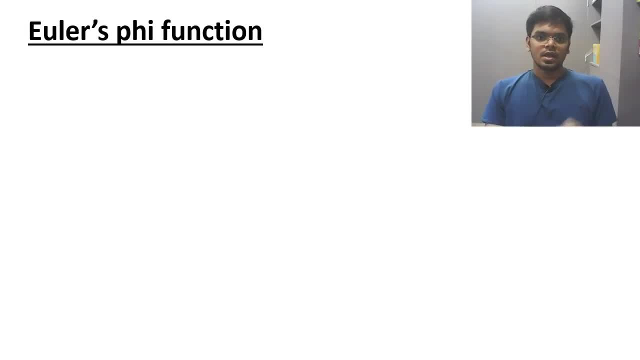 So today our topic is Euler's phi function. Now this topic can be understood better if I give examples rather than formula list, and one by one example. So I will start with the example first and I will show you how to think and how to apply Euler's phi function. So example number one: Please write it down if you are making notes. 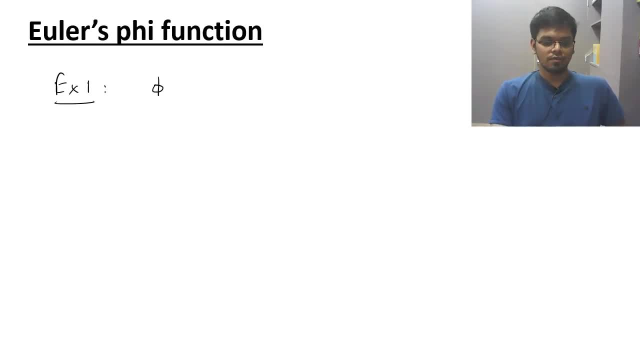 So example one is find phi of 13.. So the very first question you have to ask yourself is: what is this number? Is this number a non prime number or it is a prime number? If it is a prime number, then you can use the formula: phi of a prime number is equal to p minus 1.. 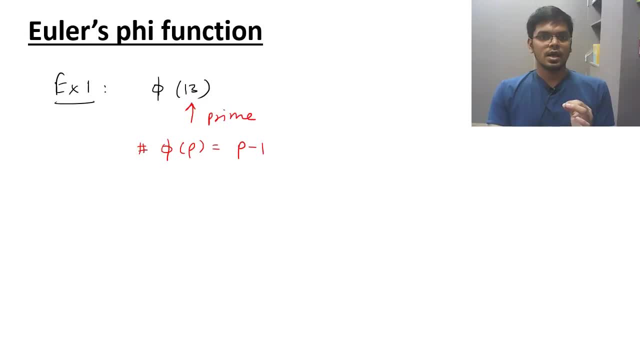 So this 13 is a prime number, correct? and the answer should be: phi of 13 is equal to 13 minus 1, which is 0.. is equal to 2. okay, so this was the example 1, where we had the prime number. now the question is what? 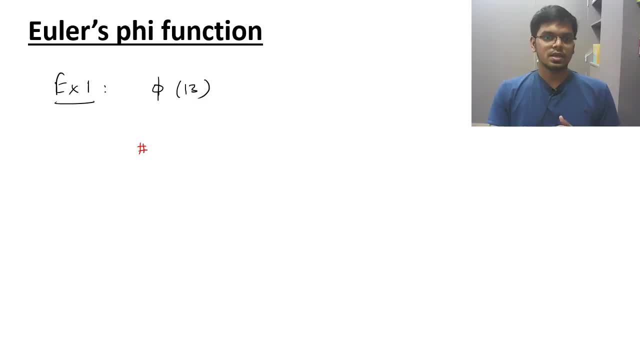 if i have a non-prime number, okay. so the example is: find the value of 5 of 10. so now this number is a non-prime number. okay, whenever you have a non-prime number, you can split the number. okay, i can write 10. okay, i can write 10 as 5 into 2. so i have splitted them into the prime numbers. 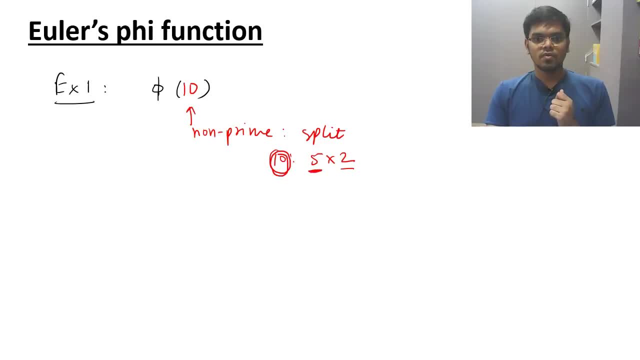 correct, i have converted this non-prime into form of a prime numbers. okay, so you can say: step number 1 conversion. okay, i have converted, and now i can write 10 as 5 into 2. now, the second point is using the euler's phi function property. the property is phi of m, cross n, okay, is equal to phi of m. 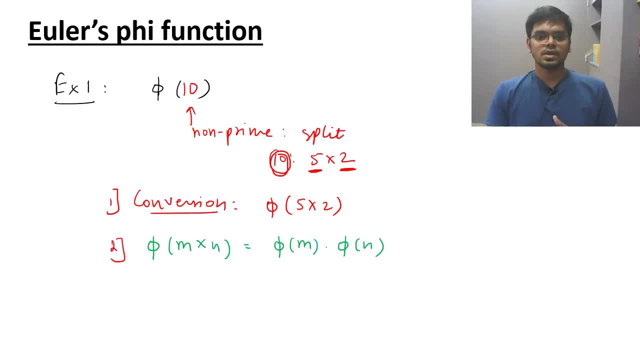 into phi of n. okay, so if this is the property, i can write the above equation as phi of phi into phi of 2. now this two values can be found from the example 1. help, okay, this was example 2. please make a note. this is example 2 in example 1. i have told you. if you want to find, 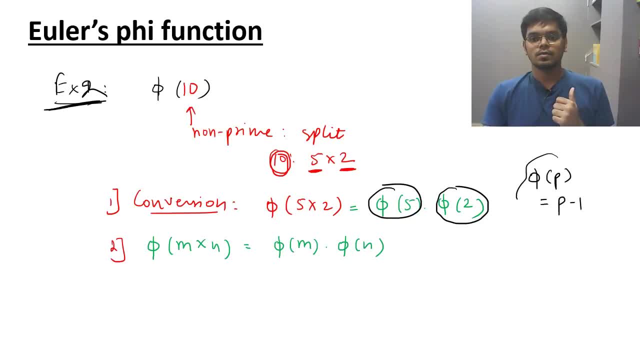 phi of p. the answer is p minus 1. okay, so apply that concept here. answer is what? phi minus 1? phi minus 1 into 2 minus 1, which is 4 into 1. the answer is 4. i hope you got the point. so up till now we have studied almost two properties. 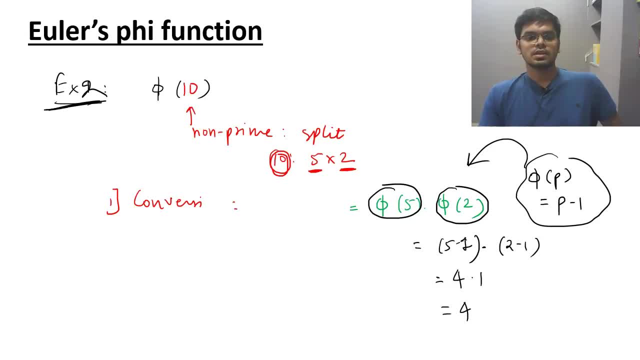 of euler's function. the first property is: if you want to find phi of p, which is phi of a prime number, then the answer is p minus 1, and if you have two number, like if you have a non-prime number, you can write that in the product of prime number form correct, and if you have a phi of m into n. 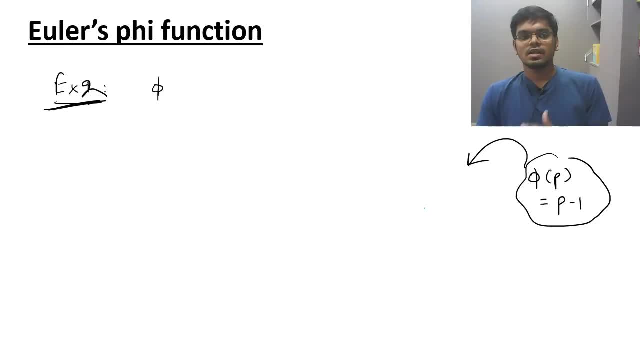 then you can split it like phi of m, into phi of n. that was seen in example 2, okay, so i hope you got the points. i will again write that property, property number 1 and property number 2 here, okay. so phi of p is p minus 1. 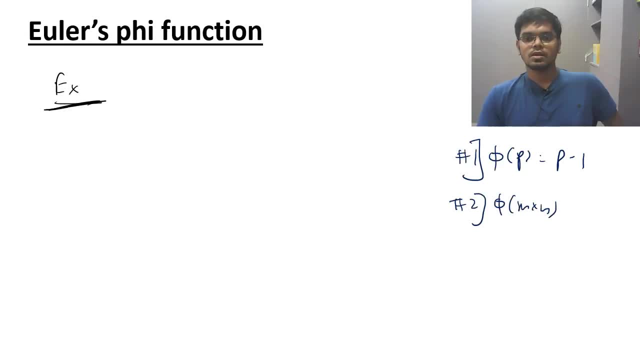 property number 2: phi of m. cross n is equal to phi of m into phi of n. now comes one more point. now, this is example 3, very important example. what if i have phi of 2, phi of p? now how to find this value? for that you have to convert this form 240. it's a non-prime. 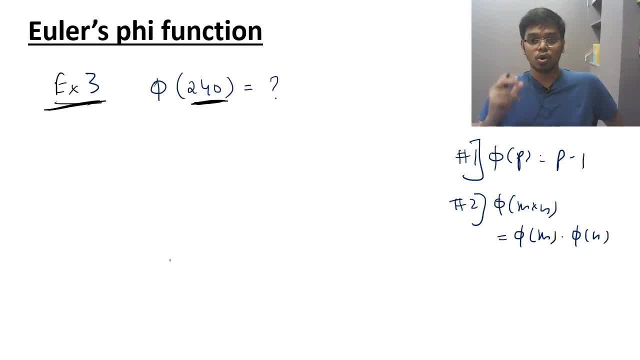 number correct. you have to convert in the form of prime numbers like product of prime numbers. for that you have to do some division. okay, so let us do the division 240. i can divide it by 2, so 2, 1s are 2, 2s are 4 and then 0. okay, then 2, 2, 6s are 12, then 0. 2, 3s are 6, then 0. 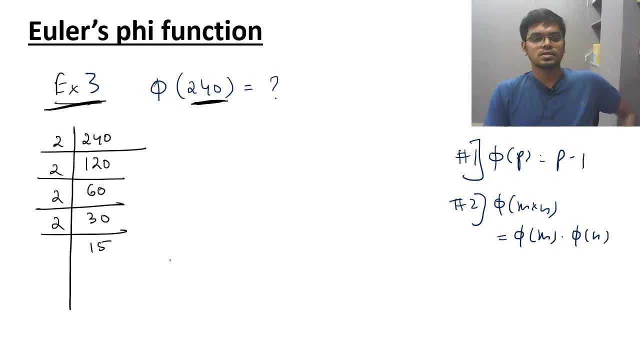 2- 1s are 2, then it would be 10. so 2- 5s are 10. now 2 is gone. now this number can be divided by 5. so 5- 3s are 15, and this is 3. so 3- 1s are 3 and you are done, okay, so this is how you have. 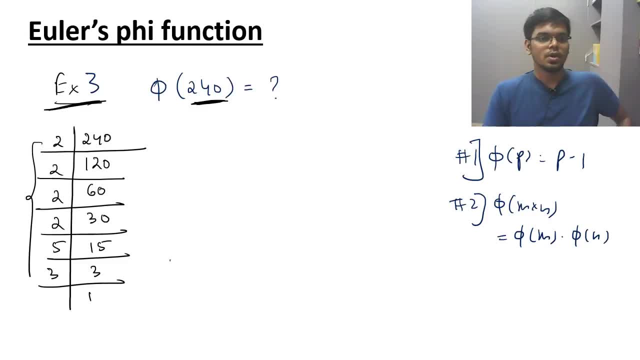 splitted your non-prime into the products of prime. so i can write, i can club, right, i can club all this- 2 and i can say it would be 2 to the power 4. okay, then we have 5, then we have 3, so this: 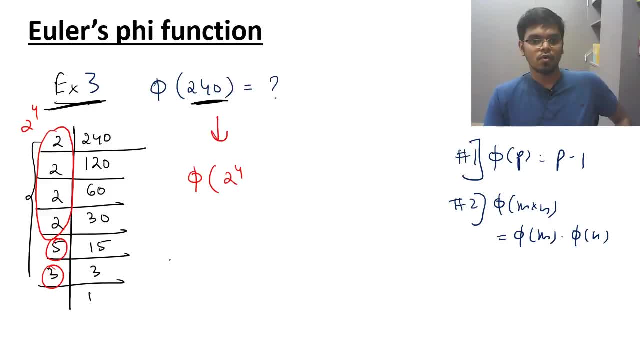 form can be written as: 5 of 2 the 2 to the power of 4 into 5 to the power 1 into 3 to the power 1. using the second property, i can split the terms. it would be 5 of 2 to the power 4 into 5 of 5. 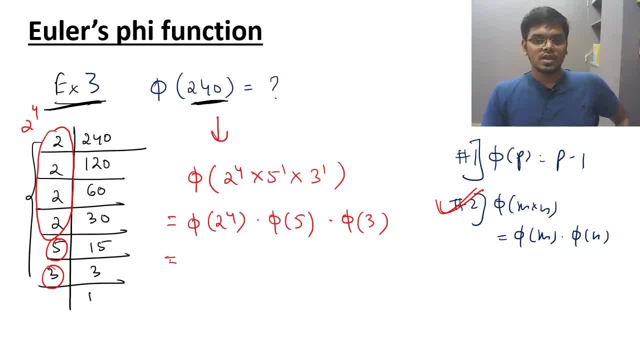 then 5 of 3. okay. now there is a problem. what to do with this term, this term? you don't know how to deal, whereas you know how to deal with this term. okay, how to deal with this term. use property 1. answer is 5 minus 1, 3 minus 1. now the first term. you have one more property, okay, so i will rub this. 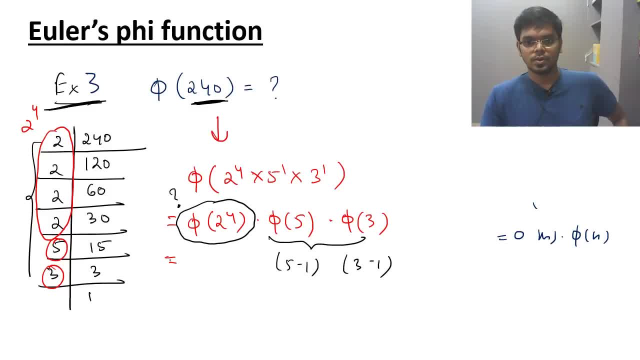 old property and i will make some space for new property. so the property number 3. the property number 3 is: if you have 5 of the prime number raised to some power, okay, which is e, then the answer is p raised to e minus p raised to e minus 1, okay, i. 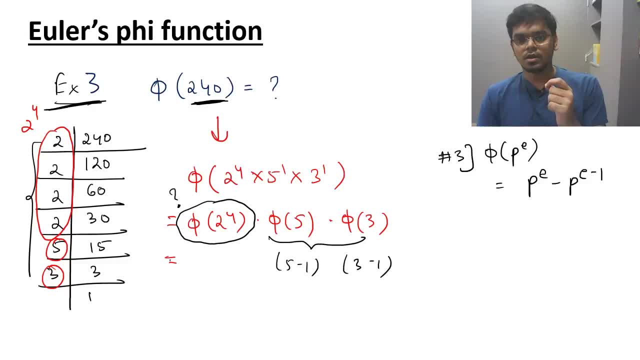 repeat, 5 of the prime number raised to power, which is p raised to e, is equal to p raised to e minus p raised to e minus 1. so this is the term where the value of p- value of p in this question- is 2 and the power e is 4. so substitute this value here. you will get 2 to 2 to the power 4. 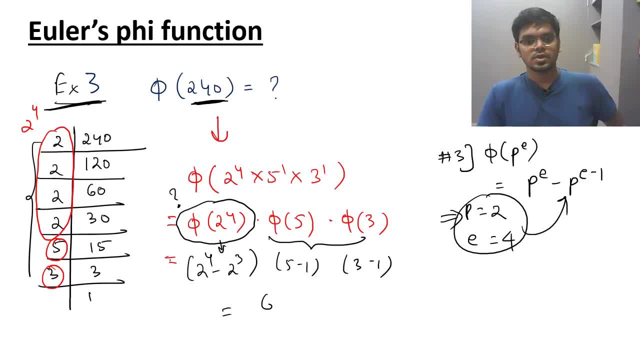 minus 2 to the power 3 and after the calculation the answer comes out to be 64. so this is example 3 of a unique variety. so i hope the three examples are clear. the first example was very simple: phi of a prime number. the second example was phi of a non-prime number in the simple way. okay, in the 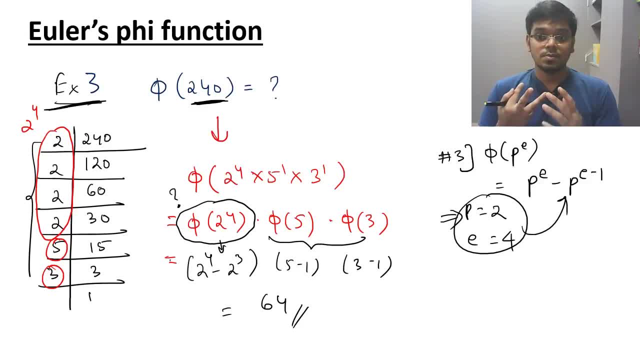 simple calculation, okay. the third example was a little bit lengthy, where you can see the number is big when the non-prime number is big, then you have to do this kind of calculation. so three properties are clear. now there is one mistake, which would be example 4. okay, so let me see how. 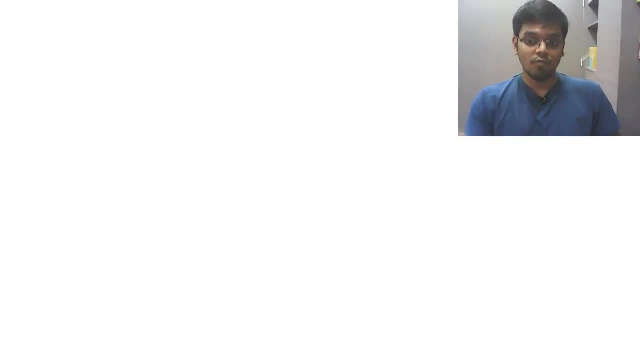 many students make that mistake and how many students make that mistake and how many students avoid that mistake. okay, so the example number four is here. example number four is find phi of 49. what is the answer now here? maximum student will do: okay, 49. it can be written as 7, 7s of 49 and 7. 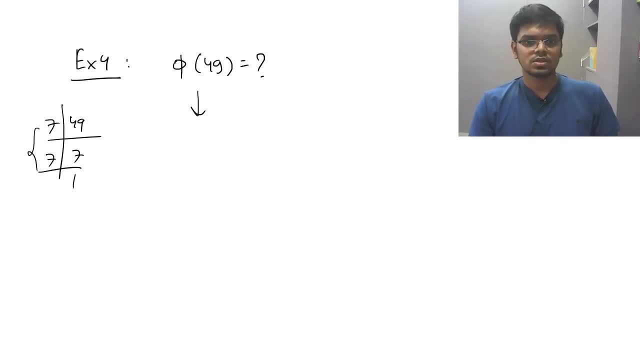 ones are okay. so 2 times 7. so this term would be splitted as phi of 7 into 7 and i can use the what was the property? phi of 49, for which we have given a property that is 7 and we have n cross. n is equal to pi of n into pi of n, So I can split it pi of 7 into pi of 7.. Then I can use: 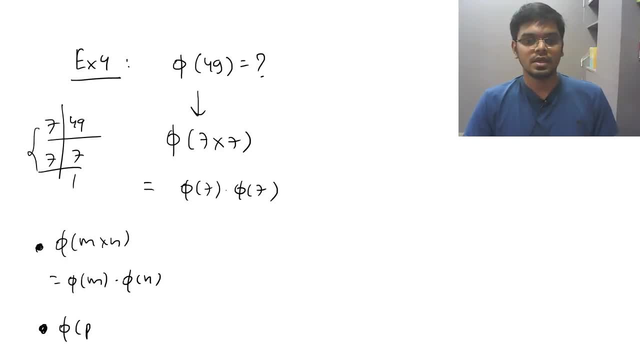 the next property. The next property is: pi of p is equal to p minus 1.. So answer would be 7 minus 1 into 7 minus 1.. It comes out to be 6 into 6, which is 36, and this is absolutely wrong. Why it is? 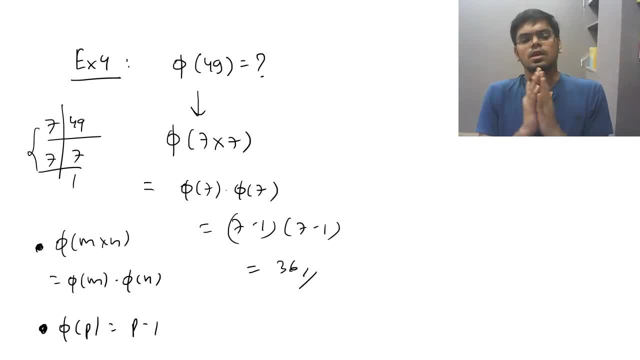 wrong. Just think, Wait a second and think. The mistake I have made here is I have split the same prime number, like 7 into 7. Whereas I have told you you have to club the prime numbers if they are same: 7 to the power 2.. You have to write that form: 7 to the power 2, which means it is of the 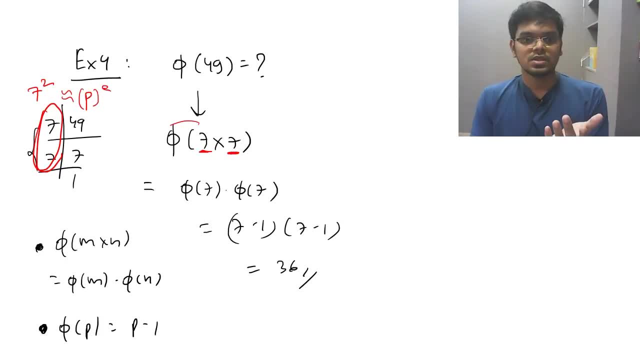 form p to the power e, And you made the mistake here: 7 into 7.. And then you use this formula. This is also. you have to take a special care. This m and n are different. m is not equal to n. Then only we can use this formula. 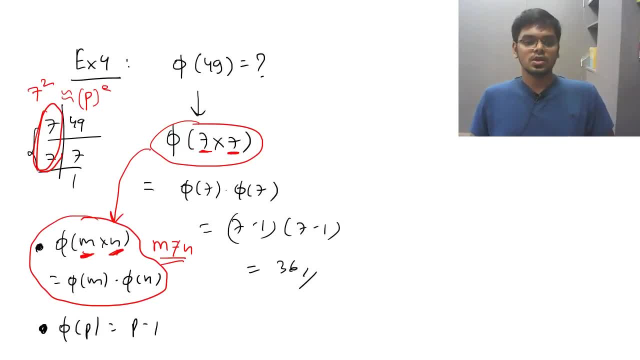 When m is not equal to n, then only we can use this formula. So this was the biggest mistake students make in the exam, So make sure you are not making that mistake. So I will erase all this part because it is wrong. You have understood that m should not be equal to n. Then only we. 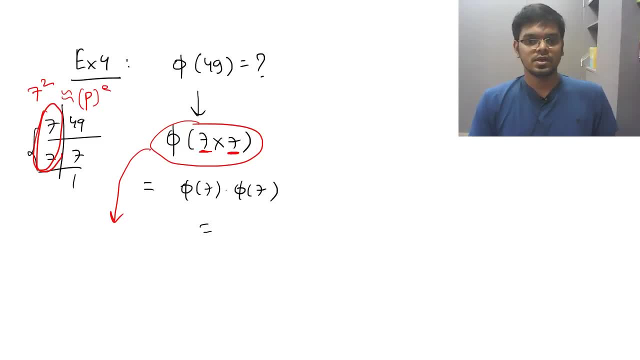 can apply the formula. So all this formula we cannot apply here, which we did earlier. So this is wrong. So what we have to do is we have to club the common part. You can see we have clubbed 7 to the power 2.. So I can write this now: 5 of 7 to the power 2.. We can use the formula. 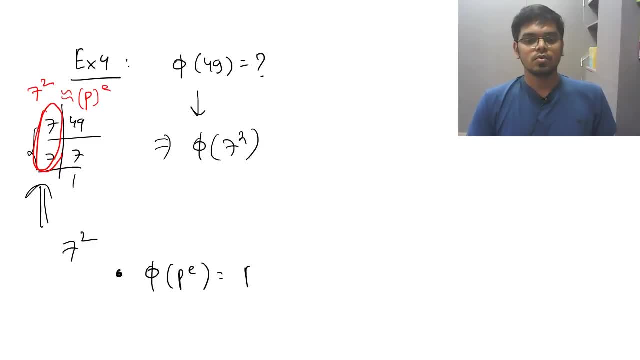 5 of p to the power e is equal to p to the power e minus p to the power e minus 1.. So the answer is 7 raised to 2 minus 7 raised to 2 minus 1.. The answer comes out to be 7 square minus 7.. 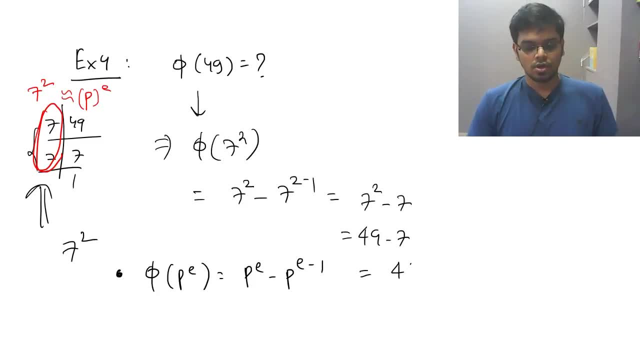 49 minus 7.. So the answer is 42.. I hope you got this point. It was very simple if you know the right calculation. So that's it for today. I have covered four examples- and the four examples are extremely important- where you have studied the complete Euler's formula. I will write all the 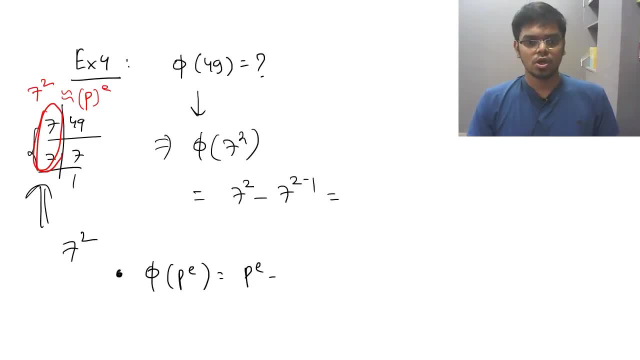 formula once again and I will give you one more note so that you can apply that also in your exams. So there are actually four formula. The first formula is: 5 of p is equal to p minus 1.. Second formula is 5 of m cross n is equal to 5 of m into 5 of n. 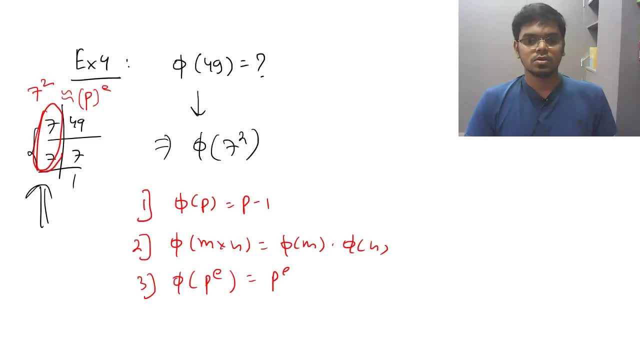 The next formula is 5 of p to the power e is p to the power e minus p to the power e minus 1.. And the fourth formula is unique. It's not used in this example, but it's unique. The formula is 5 of 1.. It's equal to 0.. So question can be like: tell me. This is the example. 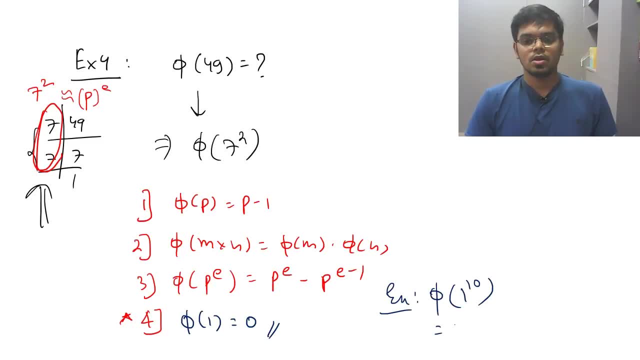 Find 5 of 1 raise to 10.. So what is the answer? So what should be the answer? The answer is 0. I hope you got this point. There is one homework question for you. The homework question is written here: Do? 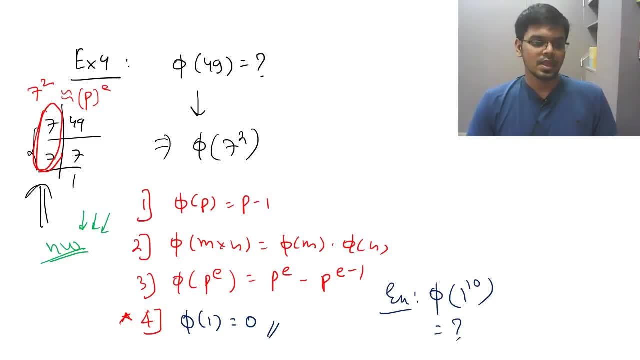 comment the answer Always. comment the homework question. You have to find 5 of 777.. Yes, You have to find 5 of 777. So do let me know in the comment section what should be the answer. That's it for. 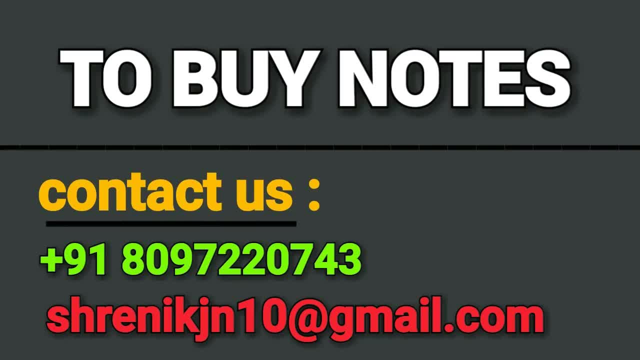 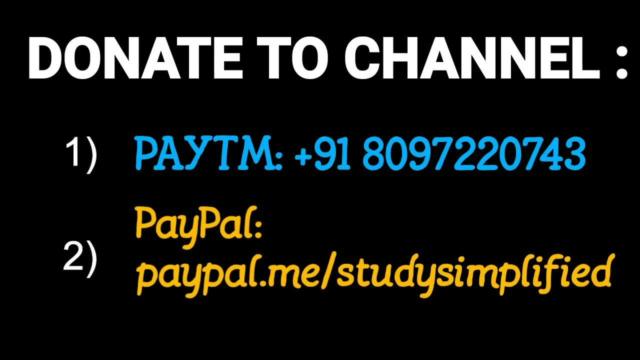 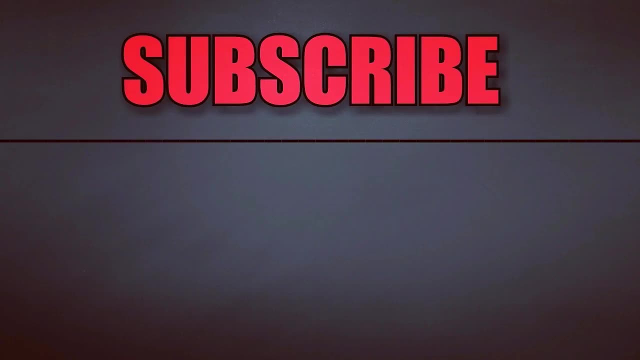 today. Meet you in the next video, Take care. So, friends, if you are liking my video, then do like this video, share with your friends and subscribe to my YouTube channel. So meet you in the next video. Till then, take care. This is Shrenik Jain. Peace out.